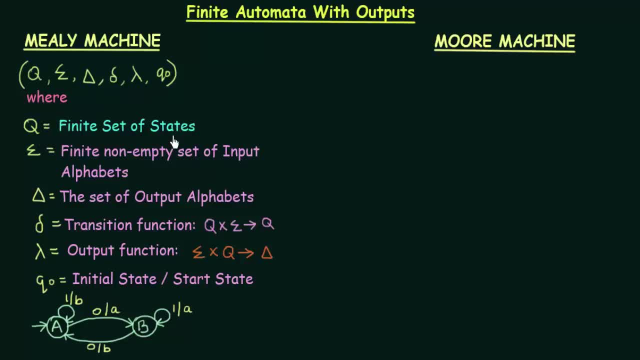 So let's see what these tuples mean. Q is the finite set of states. So this is same like our DFA, where Q is the set of states that we have And Sigma is the finite, non-empty set of input alphabets. 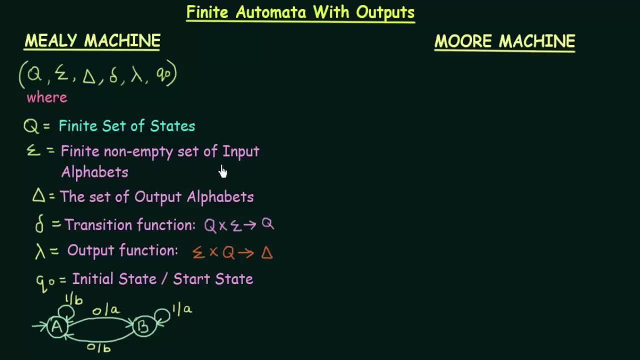 So this is also same like before, where Sigma is the set of input alphabets And Delta is the set of output alphabets. Now, this is the new thing and something different that we see. So, as I already told you, now we are discussing finite automata with outputs. 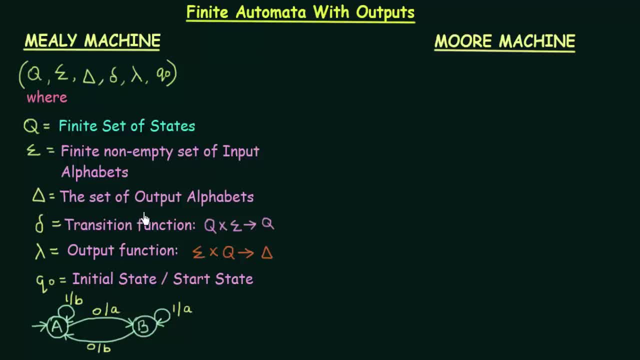 So Delta defines the set of output alphabets that we have, And Del is the transition function that maps Q, cross, Sigma to Q. This is also same, like the DFAs that we discussed And Lambda. Now this is again something different. 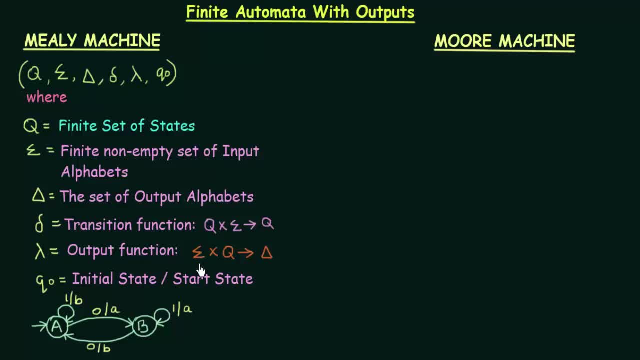 Lambda is the output function that maps Sigma, cross, Q to Delta. Now, what does this mean? This means that the input of this Mealy machine, it will be associated or it will be defined by the state that it is currently present and the input symbol associated with that state. 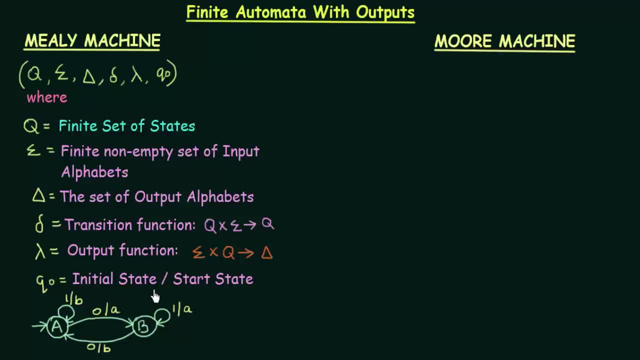 Okay, So this will become clear to you when we see the example. So, and Q0 is the initial state or the starting state. So here we have the example of a Mealy machine. So let's see, Here we have A as a starting state. 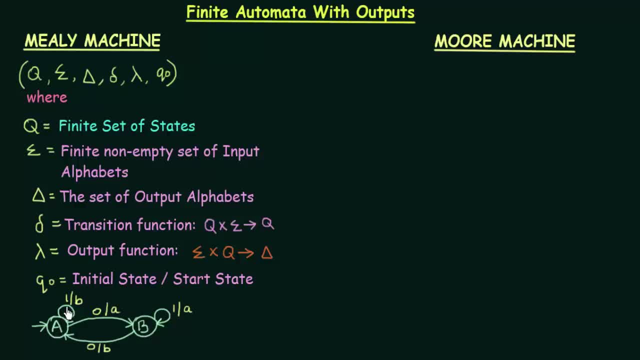 And we have another state: B And A. on getting input 1: it goes to A itself and it produces the output B- Okay. And A. on getting input 0: it goes to B and produces this output small. a And B on getting input 1. 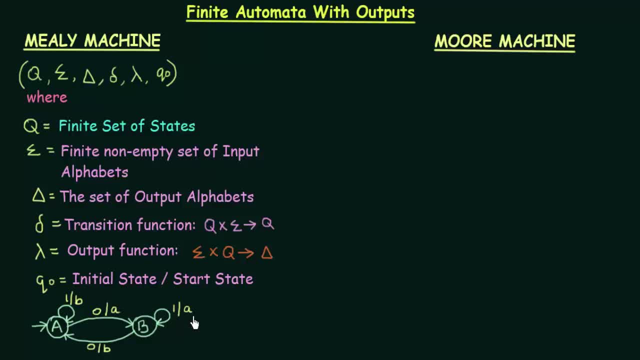 it stays in B itself and it produces output small a And B. on getting input 0, it goes to A and produces the output small b. So we see that there are outputs associated with each input and the kind of state they are present in. 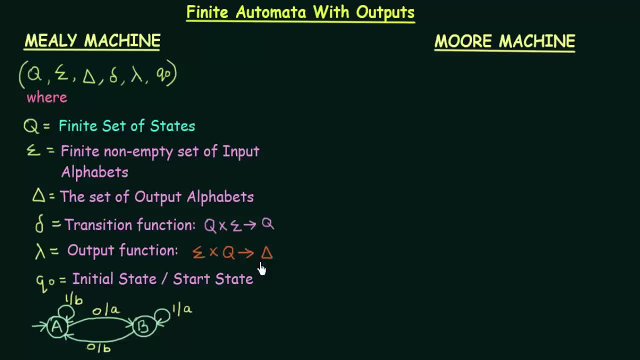 So here we said that the output function is defined by this. So the output is defined by the input and the current state it is associated to. So let us look at this example and see this output: small b. How is this small b defined or how do we get this small b? 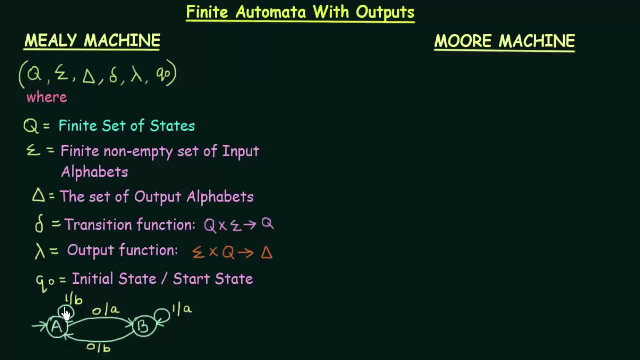 We get this small b when we are in state A and get the input 1.. So this B is defined by the state A and the input 1 that it receives. Okay, So let us see another example over here. Let us see B and let us see this output A that we get here. 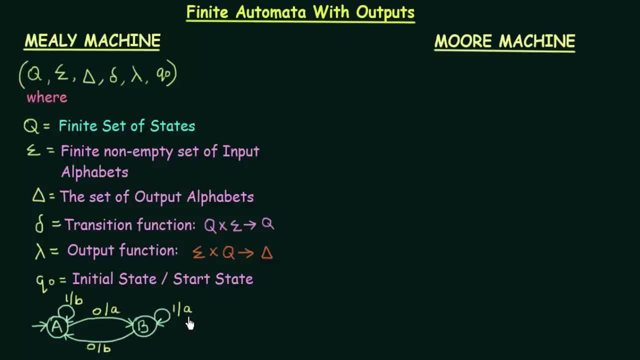 How do we get this output A? We get this output small a when we are in state B and we get the input 1.. So we see that the output is always associated to the current input that is present in the current state. Okay, 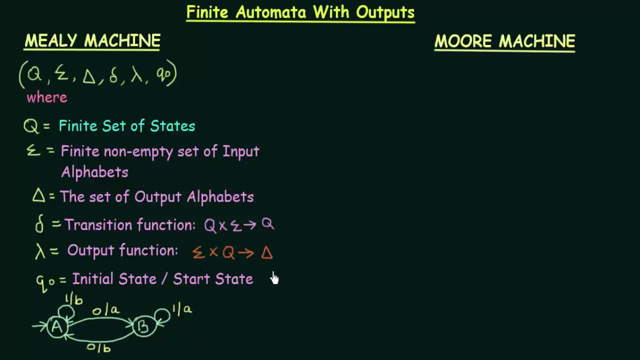 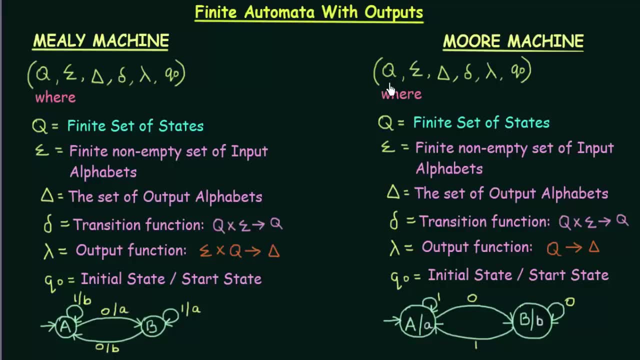 So that is how the output function of a Mealy machine is defined. Now let us go to the next one, that is Moore machine. So here we have our Moore machine, and in Moore machine it is also defined using six tuples: Q, Sigma, Delta, Del Lambda and Qnon. 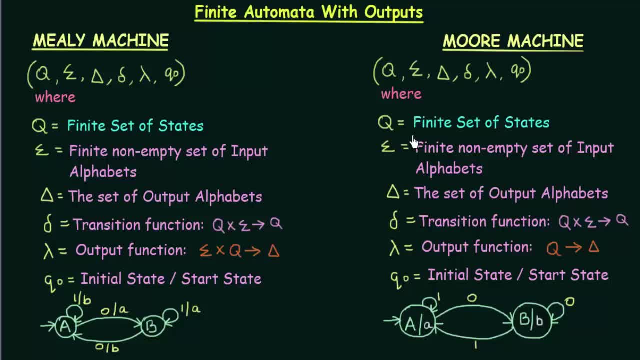 So let us see what these tuples mean. Q is the set of states, same like before. Sigma is the finite, non-empty set of input alphabets. So that is also same. And Delta is also same, like this one, the set of output alphabets. 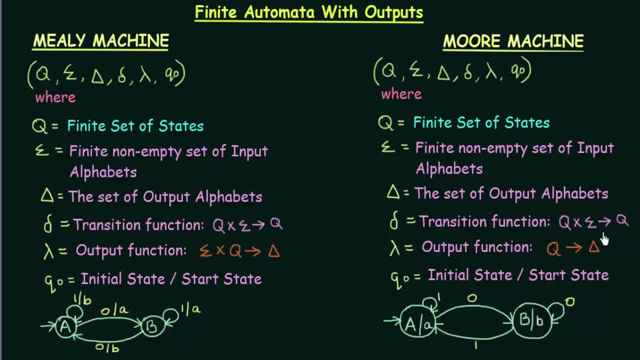 And Del is the transition function that maps Q, cross Sigma to Q. Again that is same. And Lambda is the output function that is defined by Q to Delta, And Qnot is the initial state or the starting state. So we see that the difference between Mealy machine 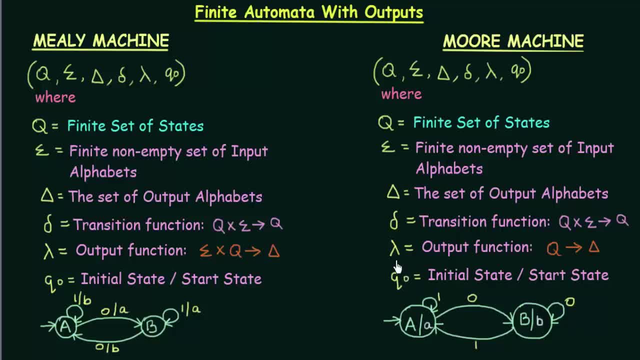 and Moore machine are these output functions Lambda. So if you look here, here Lambda was Sigma cross Q to Delta, But here Lambda is Q to Delta. So what does this mean? This means that in case of a Moore machine, the output is only associated. 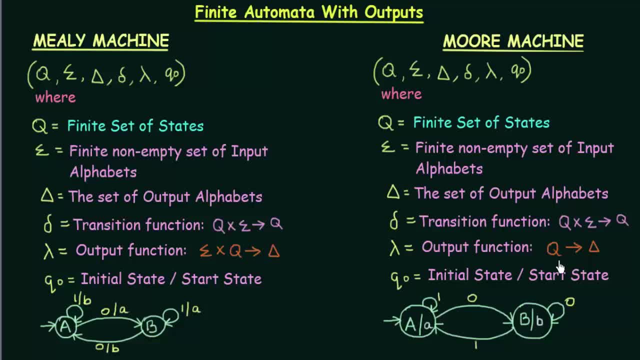 or only dependent upon the current state. Okay, this will become clear when we take this example. So look at this example. Here we have a Moore machine and here we have states A, where A is the starting state and B is another state. 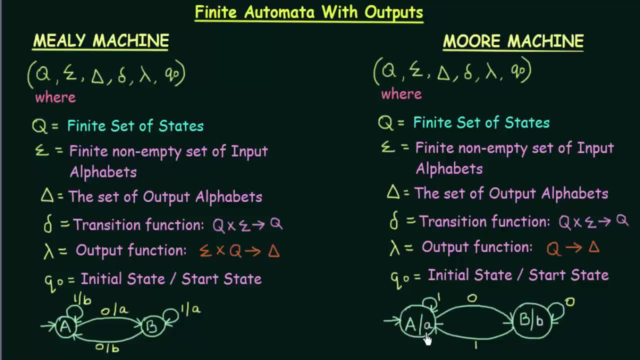 And here we see that A is associated with the output small a And B is associated with the output small b. So A on getting input 1, it goes to A itself and it produces output small a And on getting input 0,. 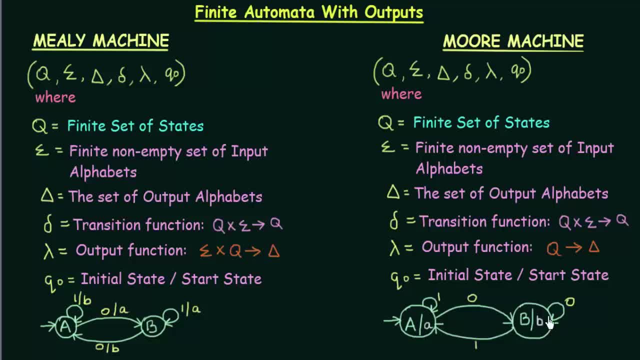 it goes to B, and this B produces output small b, And B, on getting input 0, stays in itself, producing output small b, And B, on getting input 1, goes to state A, producing output small a. So here we see that these outputs are dependent only on the states. 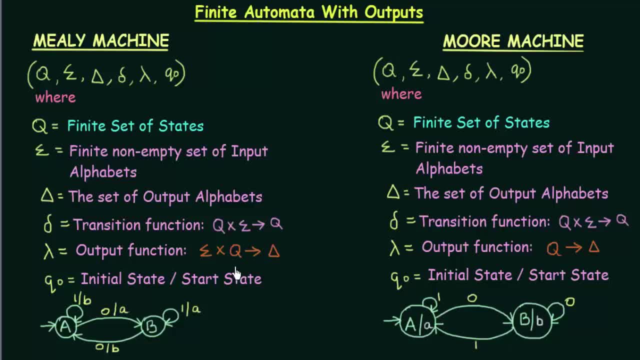 Okay, it is defined by the states. But in this case, in case of Mealy machine, we see that the outputs were related or defined by the state, as well as the input that we get in that state. But here it is only dependent on the states. 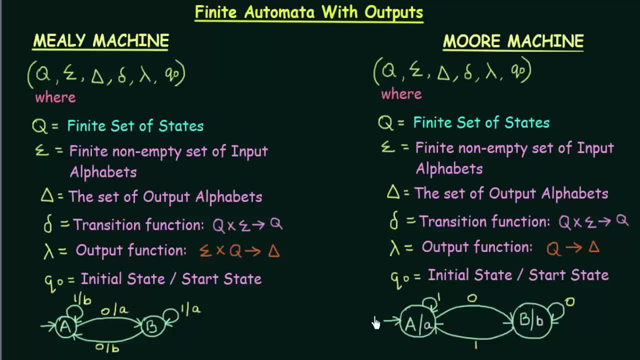 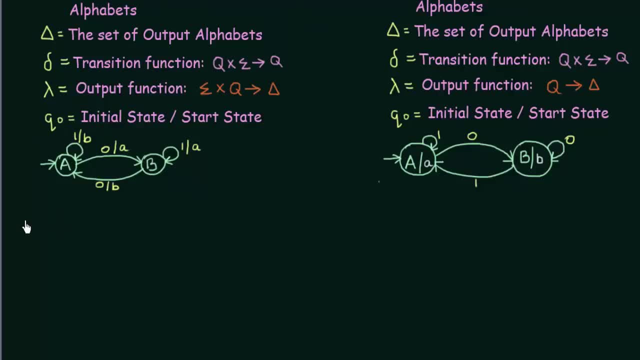 So this will become more clear when we take an example. So let us take a simple example. So suppose in my Mealy machine I am going to pass an example string, So let my string be 1010.. I am going to pass this to my Mealy machine. 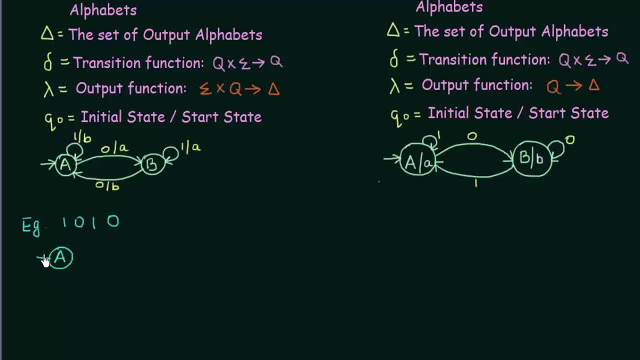 So it starts with the starting state A. Alright, it starts with starting state A And A on getting input 1, what happens On getting input 1, A goes to A itself, A goes to A itself And it produces the output b. 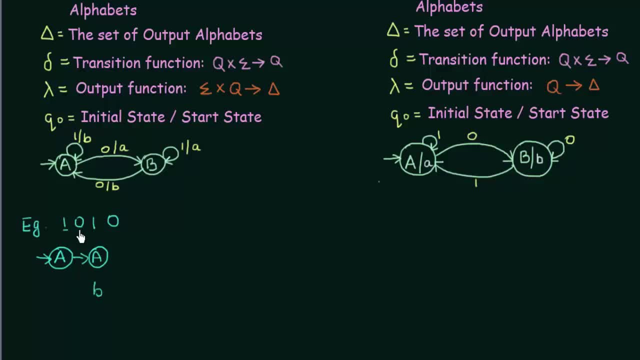 It produces output b. Okay, now we are done with this. Now come to this one: 0.. A, we are in A. now A on getting input 0, it goes to b And as it goes to b, 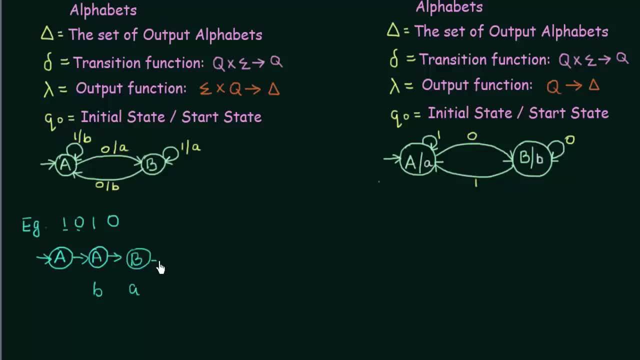 it produces output small a. And then now we are in b And the next input we get is 1.. And b, on getting input 1, goes to b itself, Goes to b itself And it produces output small a, And we are done with this. 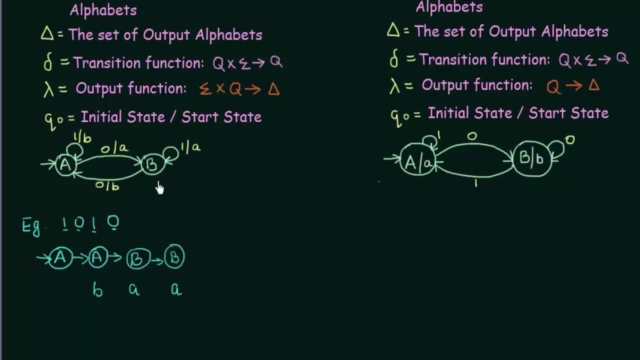 Now we come to this: We get 0 and we are in b And on b. when we get 0, it goes to a. It goes to a And it produces output small b. So b goes to a, producing output small b. 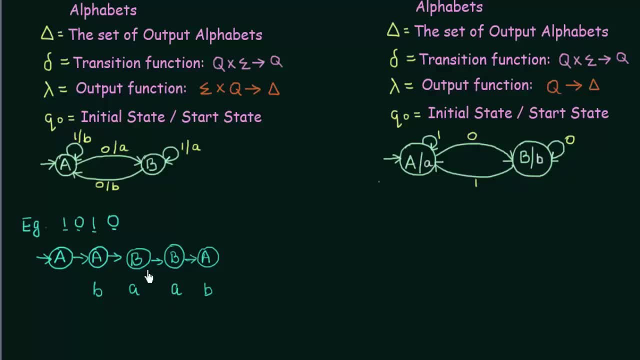 So here we get the output b, a, a, b in this mealy machine. Okay, now let's try the same example: 1, 0,, 1, 0. And let us pass it to our more machine. 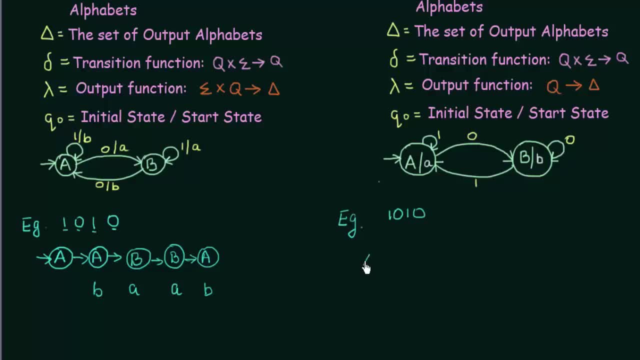 And let us pass it to our more machine. So in more machine also it starts with starting symbol a. So it starts with the state a. So it starts with the state a. And here one thing you have to notice: 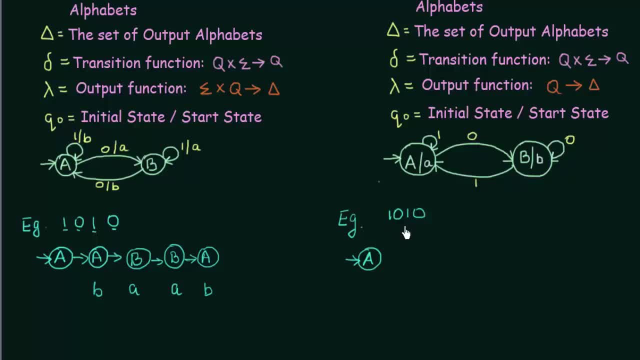 when you are in a, even before you get anything, even before you feed any input to this state, even before you feed any input to this state when you are in a output small a, So even before you feed the string. 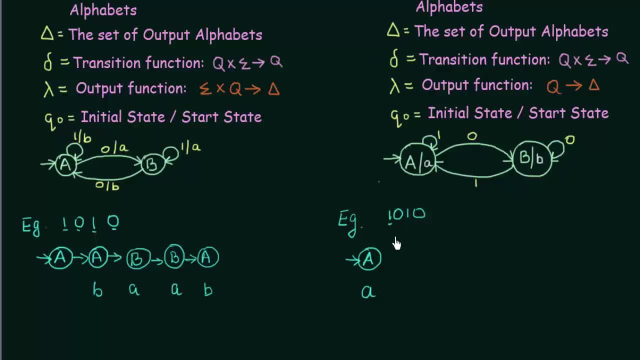 a gives the output small. a. Now we get the first input symbol 1.. Now we get the first input symbol 1.. So a on getting input symbol 1, it stays in a itself And in a it produces output small a. 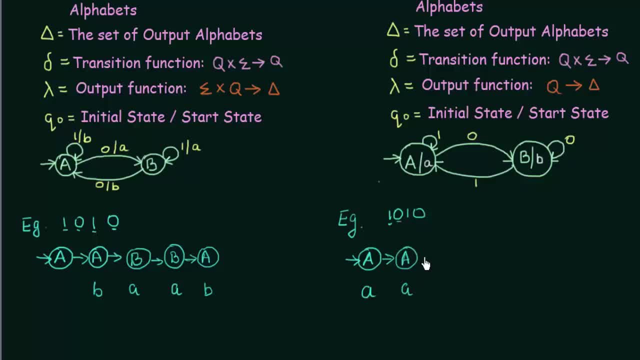 And then next is 0.. And we are in a. Where does a go on getting input 0? It goes to b, And when it reaches b, b produces output small b. Next input is 1.. And we are in b. 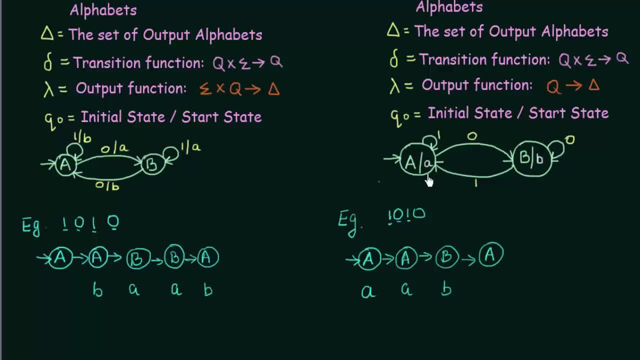 b on getting input: 1 goes to a And it produces output small a And it produces output small a. And now we are coming to the last input, that is 0.. And we are in a. a on getting input: 0 goes to b. 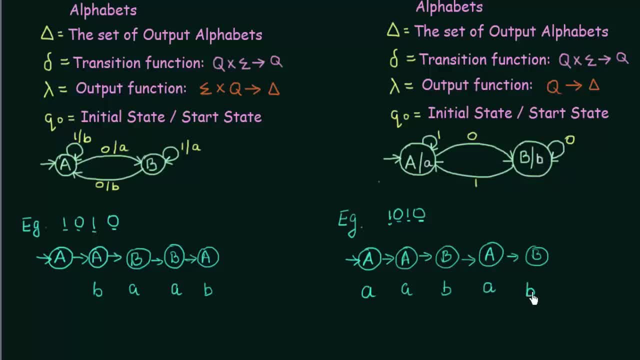 And b produces output small b And b produces output small b. So we get the output a a, b a b. So we get the output a, a, b a b. So this is how the 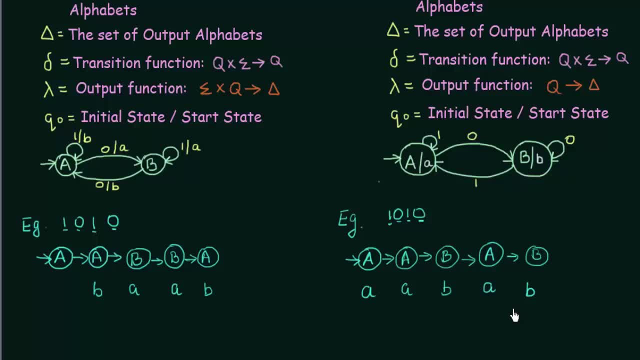 Mealy Machine and Moore Machine behave on getting certain input strings. Now, if you notice here, you see that in case of Mealy Machine, when we gave an input string of length 1,, 2,, 3,, 4, it produced an output string of length. 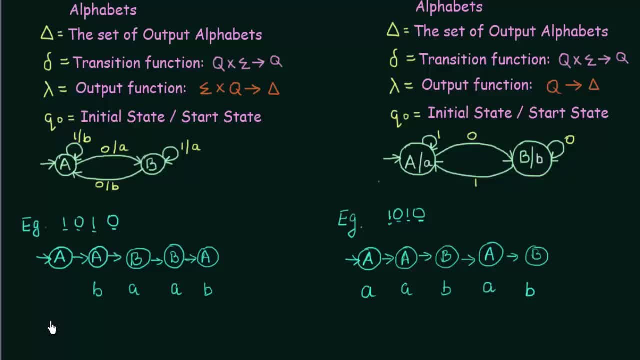 1,, 2,, 3,, 4.. So that means, if the length of your input symbol is n, then the length of your output symbol is also n. But in case of Moore Machine the length of our input symbol was 1,, 2,, 3,, 4.. 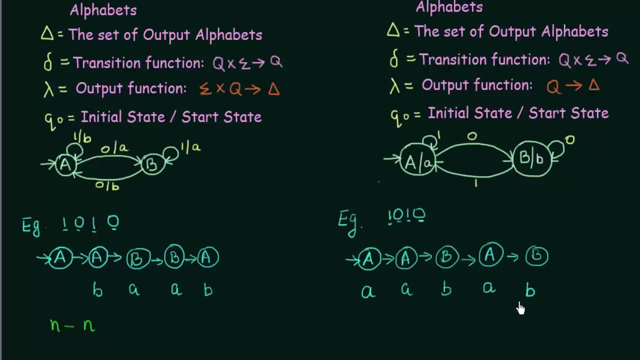 And the length of the output string that is produced was 1,, 2,, 3,, 4, 5.. So in this case we see that if the length of your input string is n, then the length of output string is always.